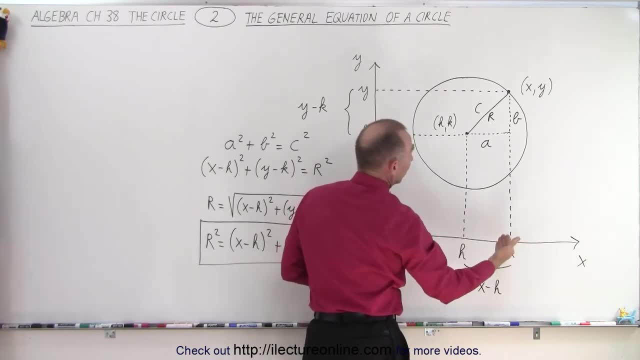 the distance a is simply a squared plus b squared equals c squared. So we can also see that the distance b is simply x minus h. irregardless where x is- You can take that point anywhere along the circle- this distance will always be x minus h. And this distance right here, no matter where. 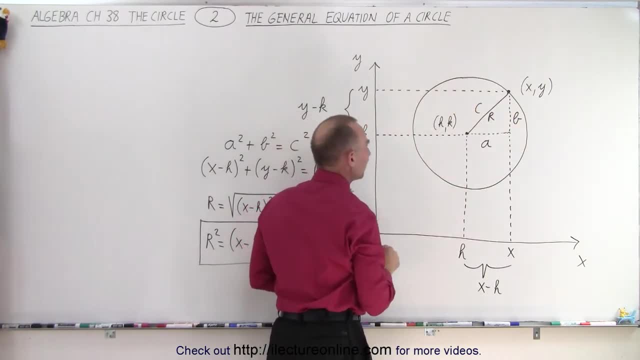 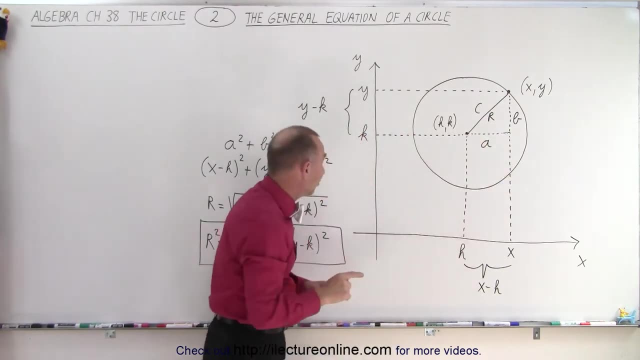 you put the point on the circle that distance will always be y minus k. Now, of course, if this point is lower than the center, then y minus k will be negative number. but it doesn't matter, since we're going to square that anyway. So negative number, positive number, it makes no. 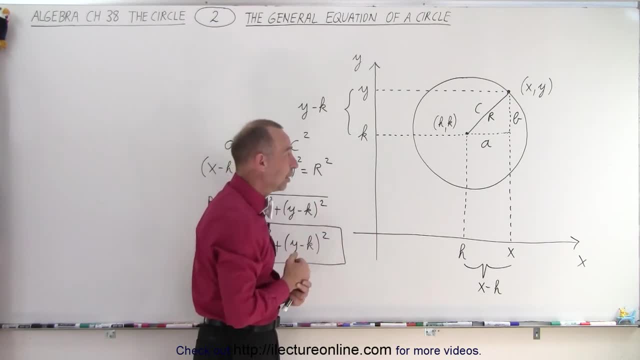 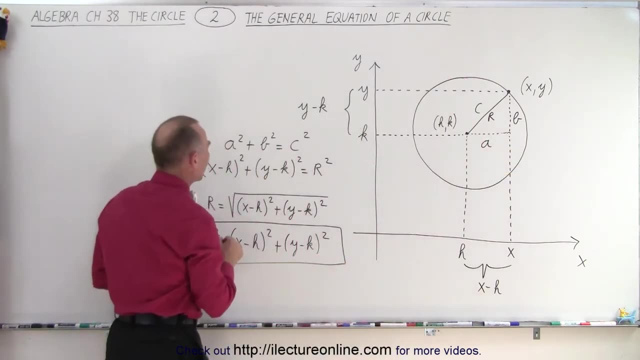 difference, since we're squaring both side a and side b, So it doesn't matter where x y is, We can have any point in the circle and this will always work. So now, instead of calling a a, we're going to call it x minus h, And instead of calling b, 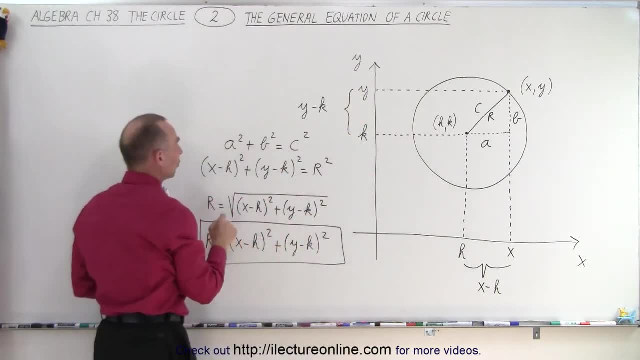 the side b, b, we're going to call it y minus k. So instead of a squared, we get x minus h squared. Instead of b squared, we get y minus k squared, because x minus h is the same length as a. 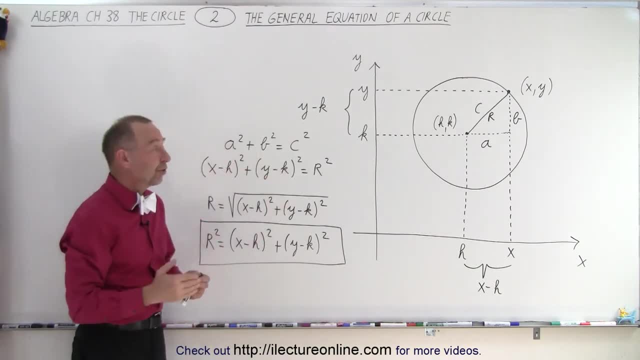 and y minus k is the same length as b, And of course the hypotenuse c is simply the radius of the circle. And then we know that x minus h squared, plus y minus k squared, equals r squared, and that's essentially the equation of a circle, the general equation of. 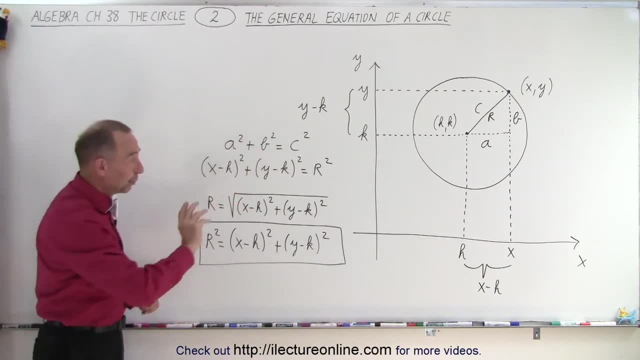 a circle, no matter where you put the circle in the x- y plane. So if we turn that equation around, we have r squared equals the quantity x minus h squared, plus the quantity y minus k squared. And of course, if you take the square root of both sides, you end up with r equals the square root. 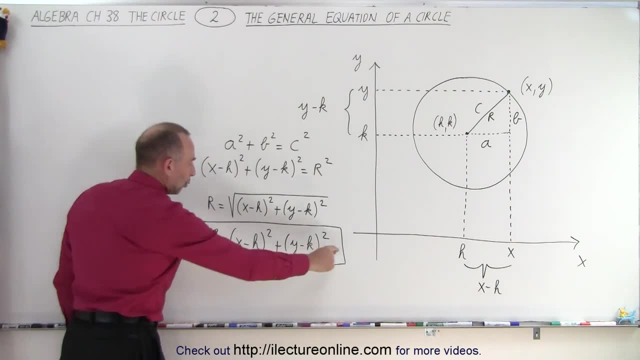 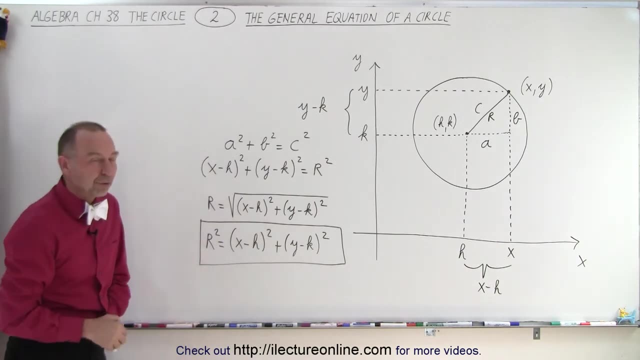 of x minus a squared, plus y minus k squared, but the real equation is the one that we boxed in. later on we'll see what this, what essentially the difference is when we think about it in terms of algebra. but there it is the general equation of a circle. no matter where you place the circle. 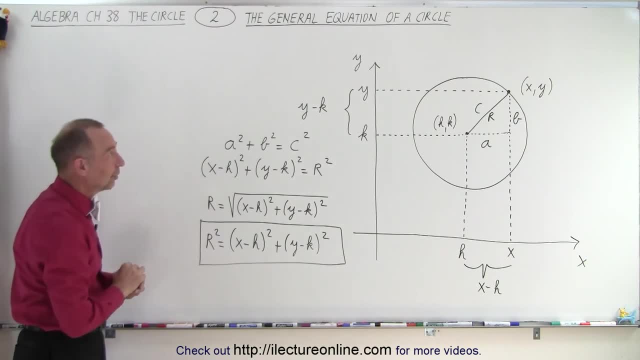 no matter the size of the radius or where the location of the center is, this will always represent the general equation of a circle, and that is how it's done. you need a nap really bad, all right, see, now you know why it's: it's related to the distance from them.